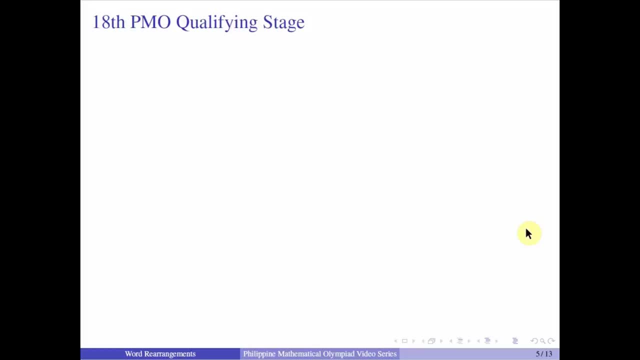 so now let us proceed with solving some problems from pmo qualifying stage. so for the first one we have part 1, number 11. in how many ways can the letters of the word qualifying be arranged such that the vowels are all in alphabetical order? so now we will be doing permutation with 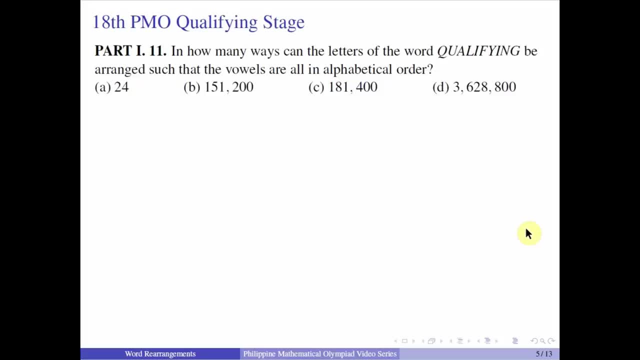 identical objects. so we classify each object into certain types. in this case, each letter corresponds to a certain type of object, so we classify each object into certain types. so you have q equals 1. l is equal 1. we have 1 f, 1 y, 1 n and 1 g, but for all vowels we will just be 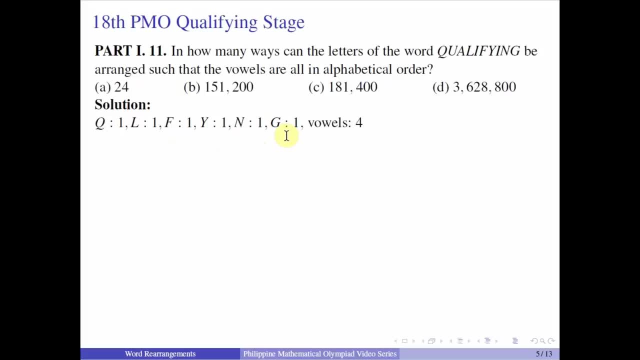 taking them as one type. so you have four vowels. so now the question is: how come all of the vowels are just considered as one type, even if some of the vowels are different? so in here you can see one u, one a and then two i. so the reason behind it is because, um, the problem wants that the vowels are. 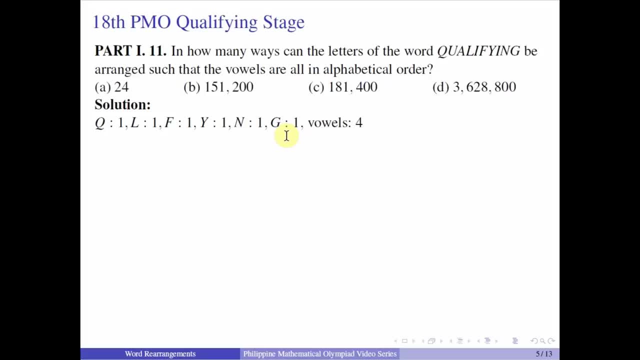 in alphabetical order. so once we choose the positions where the vowels will be filling out, then you already know how they should be positioned. it would just be um, a and then i, and then i and then u, so it's just as if all of the vowels are just the same. 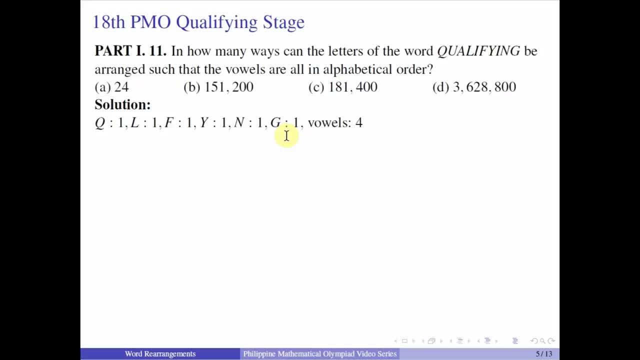 so, so there. so now we will be using um permutation with identical objects. so you have a total of 10 letters, and then so you just divide it by six i's from six different consonants, and then you have four factorial for the four vowels that we considered as. 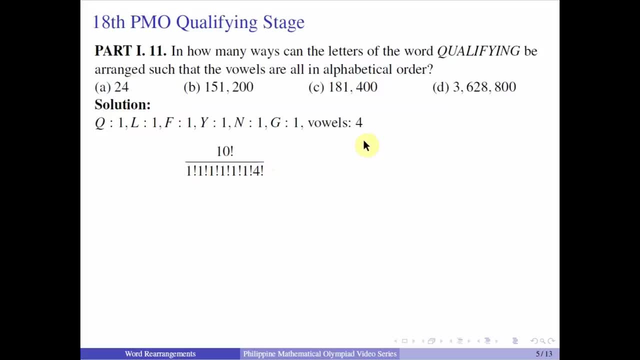 identical, and then you have a four factorial for the four vowels that we considered as identical objects. then we simplify, so we divide 10 factorial by four factorial, so we are left with five times, six times, seven times, eight times, nine times ten, so which is equal to 151, 200. so the 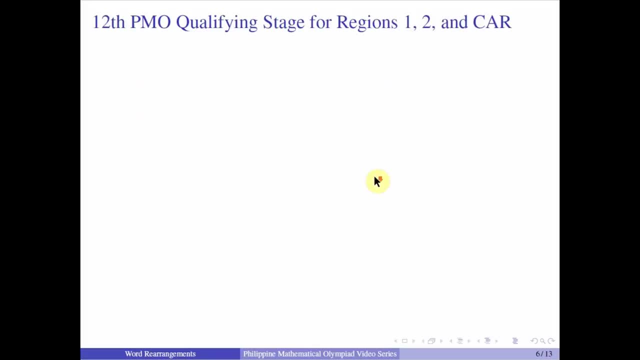 answer is letter b. now let us proceed with the 12 pmo qualifying stage for regions one, two and car new. so for part 1, number seven, in how many ways can the letters of the word olympiad be rearranged in such a way that the vowels appear in alphabetical order and the consonants also appear? 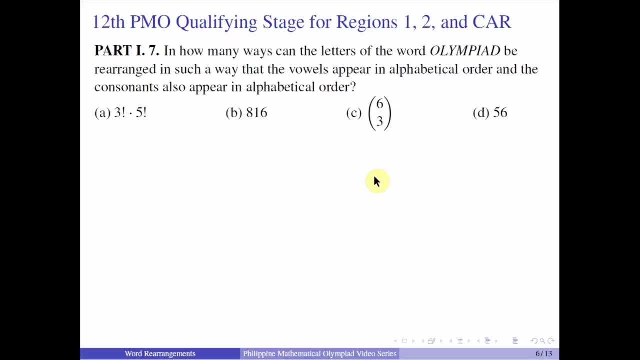 in alphabetical order. so, in the same manner as the previous problem, we just consider all of the vowels as one type and then we also consider all the consonants as another type. so you have a total of three vowels and five consonants. so you have a principle of three vowels and five consonants. 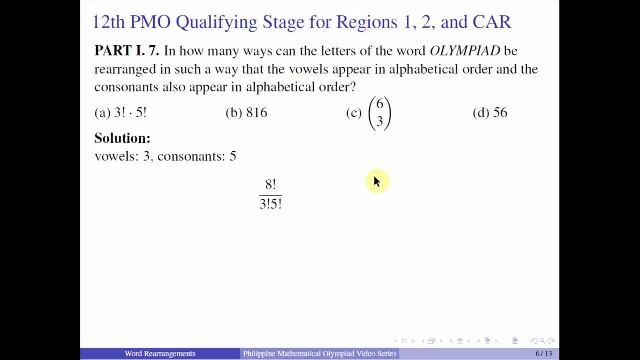 so you have a total of 8 factorial over 3 factorial, 5 factorial ways. so to simplify, you can cancel out 8 factorial with 5 factorial, so what is left in the numerator would be 6 times 7 times 8 and then on the denominator you, you have um, you can expand 3 factorial to 1 times 2. 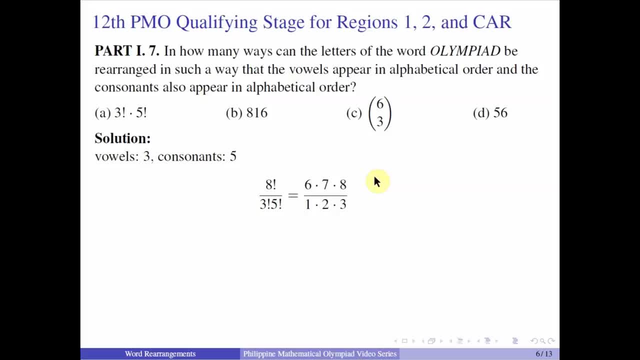 times 3, so you just cancel out 6 with 2 and 3, so you are left with 8 times 7, which is 56. so the answer for this item is letter d 56. all right, so let us proceed with next item. so from: 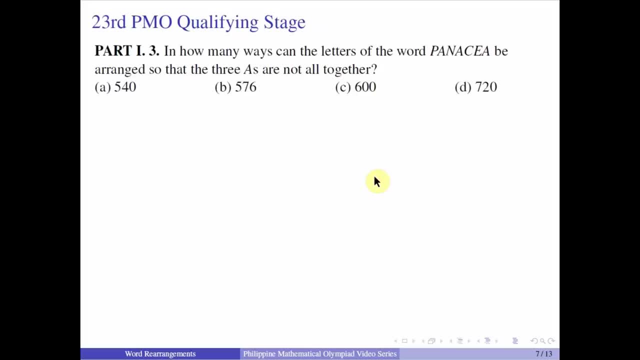 the 23rd pmo qualifying stage, part 1, number 3: in how many ways can the letters of the word panacea be arranged so that the three a's are not all together? so now, what we're going to do is first to count the number of formative. 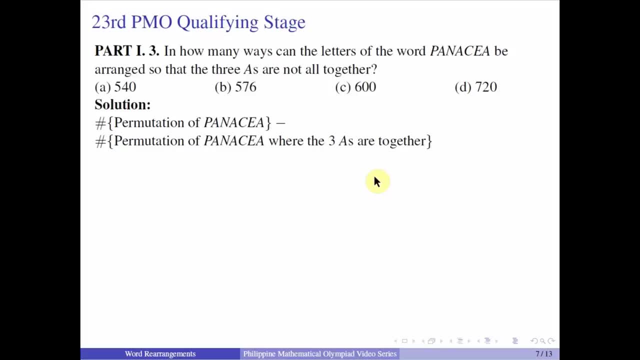 permutations of panacea, so which you can just easily use, the um, the concept of permutation with identical objects, and then we subtract all of the permutations of panacea wherein the three a's are together. okay, so to count for the number of permutations of panacea. so you just count all. 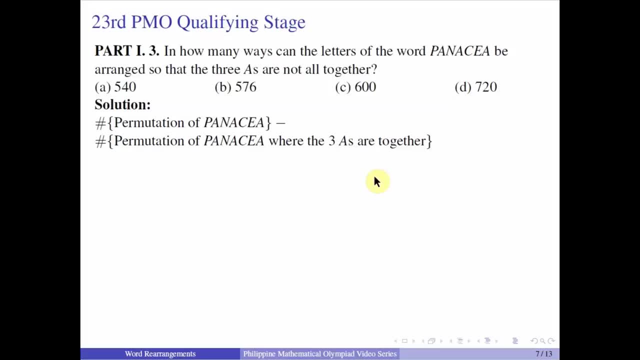 the distinct letters. so you have one p, one n, one c and one e, and then you also have three a's, so you have a total of seven letters and then you divide, so that's seven factorial all over, so you have four, one factorials and then three factorial. 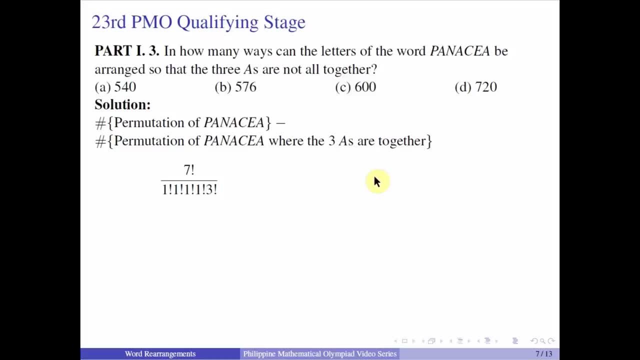 and then to count for the number of permutations of panacea where the three a's are together. so we just take all of the three a's as one object. so now you have one object, that is three a's, and then you have one p, one n, one c and one e. so you 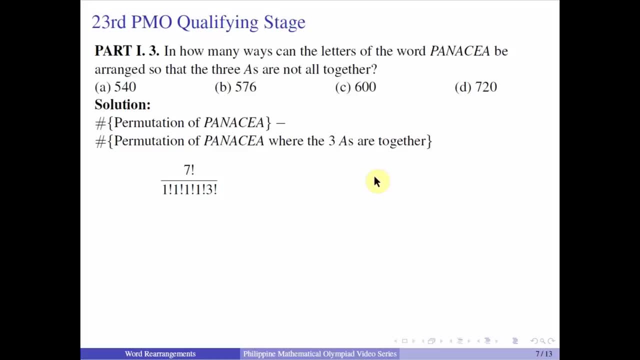 you have a total of five distinct objects. so to permute that you get five factorial, and then you just need to simplify so, um, so the first expression would just be four times five times six times seven, and then you can expand five factorial, you can factor out four and five there. 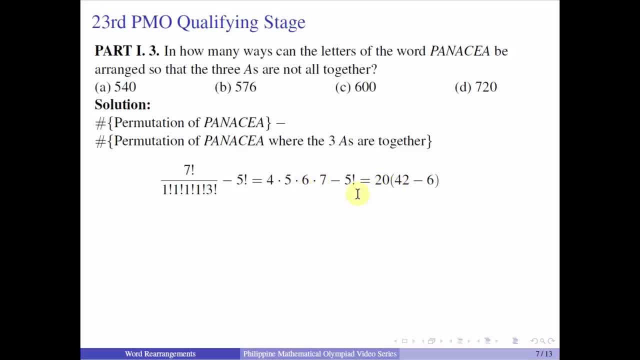 so you get 20 times. so for the first expression, six times seven is 42, and then for five factorial, you factor it out four and five, so you are left with one times two times three, which is six, so 20 times 42 minus six, so that's 20 times 36, so which is 720.. so the answer here is letter d 720. 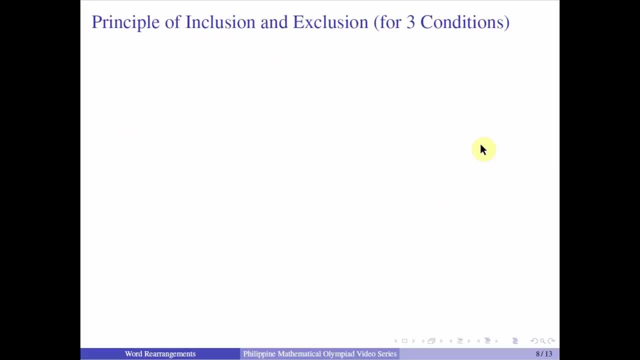 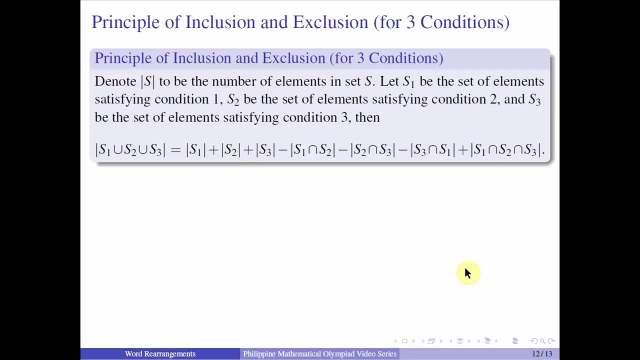 now for the last item. we will be introducing what we call as the principle of inclusion and exclusion. the cardinality of s sub 1 unis union s sub 2, union s of 3 is just equal to the cardinality of s sub 1 plus the cardinality of s sub 2, plus the cardinality 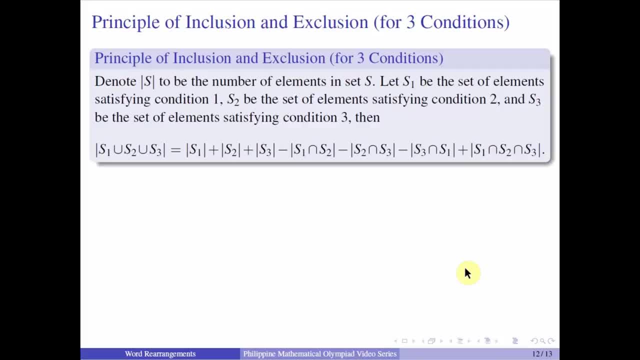 of s sub 3 minus the cardinality of s sub 1. intersection s sub 2 minus the cardinality of s sub 2. intersection s sub 3 minus the cardinality of s sub 3. intersection s sub 1 plus the cardinality. 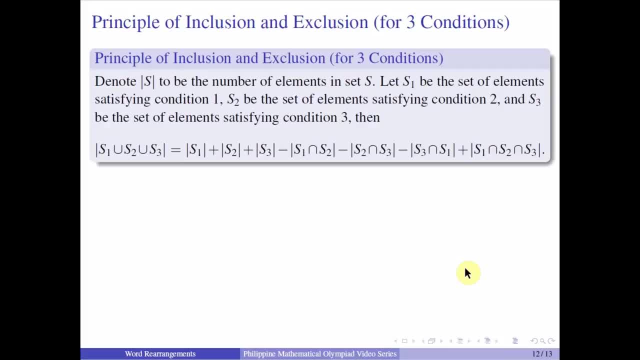 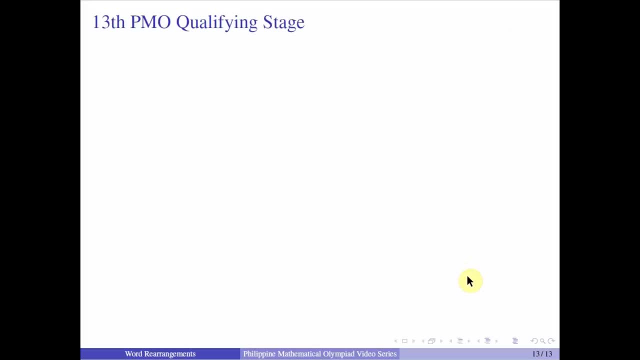 of sub 1, intersection, sub 2, intersection, sub 3. all right, so now let us proceed with the last problem that we will be discussing. so this is coming from the 13th PMO qualifying stage, part 2, number 10: in how many ways can the letters of the word murmur? 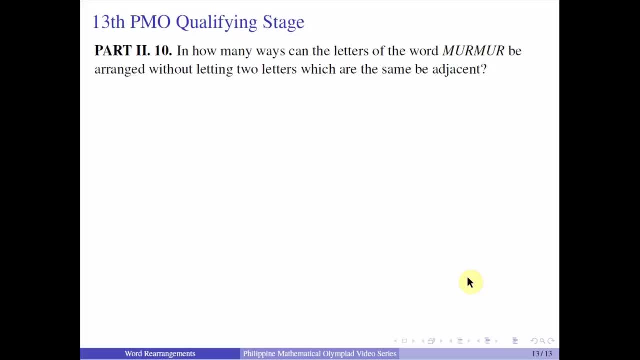 be arranged without letting two letters which are the same be adjacent. okay, so we let sub 1 be the set of permutations of murmur where the two m's are adjacent, and then we do similar conditions for sub 2 and sub 3, except that for sub 2 we want: 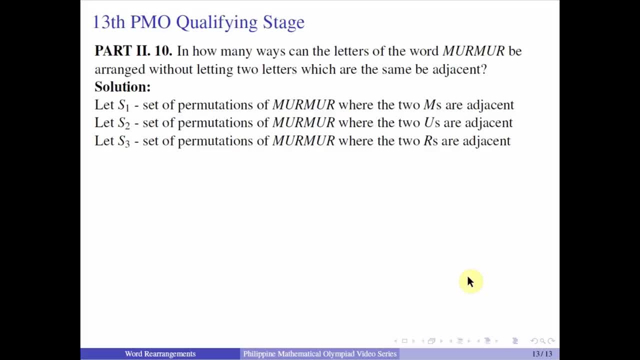 the two u's to be adjacent, and then for sub 3, we want two r's to be adjacent, and then what this problem is asking is the number of permutations of murmur. and then you subtract the cardinality of sub 1 union, sub 2 union, sub 3. 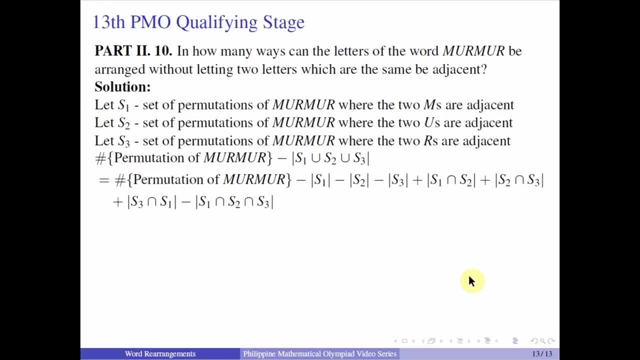 and so using the principle of inclusion and exclusion, so you have here this one. okay, so to compute for the permutation of murmur, so you just need to count the number of distinct letters, so you have two m's, two u's and two r's, so you have a total of six letters. so that's six factorial all over. 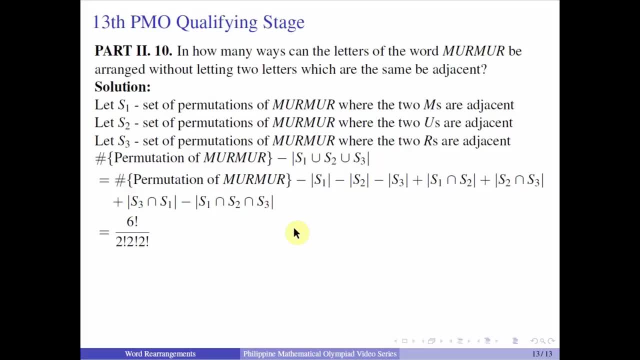 two factorial, two factorial, two factorial. so now we want to compute for the number of permutations of murmur where the two m's are adjacent. so we consider the two m's as one object, and then you have two u's and then two r's, so you have a total of five objects and then you divide it by one factorial two. 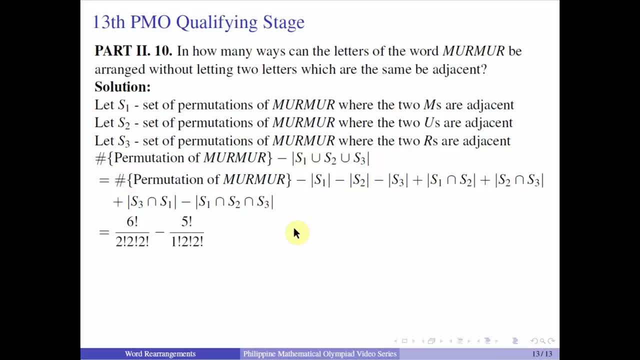 factorial, two factorial, and then you also do the same thing for sub 2 and sub 3, and then next. so we want to get the cardinality of sub 1 and sub 2, union intersection, sub 2. so in here we will be treating the two m's as one object, and then we will be treating 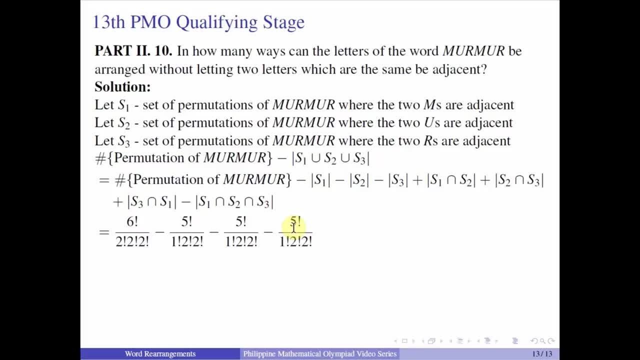 the two u's as another object, and then you have another two r's, so you have four factorial all over: one factorial, one factorial, two factorial, and then you have another two r's, so you have three factorial, and then you also do the same thing for the other two s. sub 2 intersection. 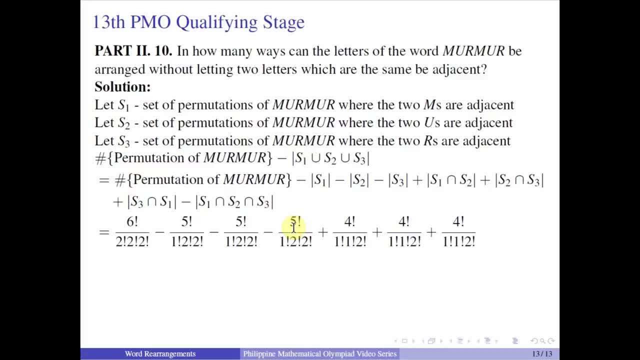 s sub 3 and s sub 3, intersection, s sub 1, and then, lastly, so we want to get the cardinality of the intersection of the three sets. so you just take the two m's as one object, you take the two u's as one object, and then you take the two r's as another object. so you have.